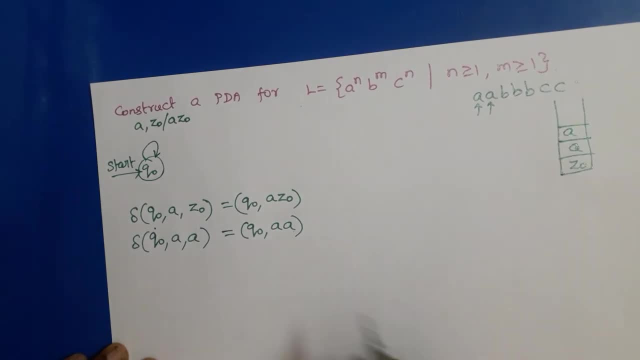 So a, a, a. another a is also pushed onto the stack. So q0 to q0, a comma, a slash a, a. Now q0 is a current state and the next input is b. Top of the stack is a Means. 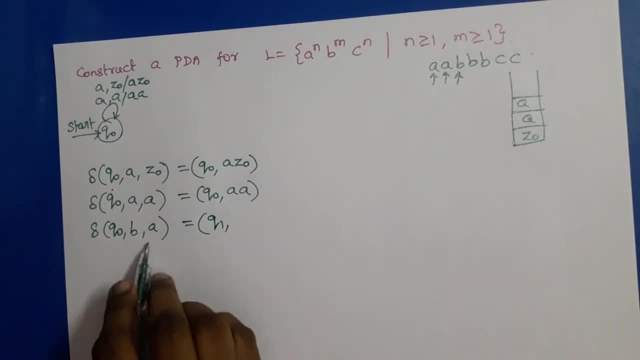 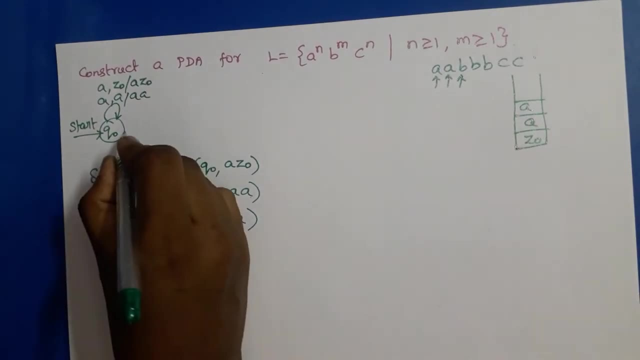 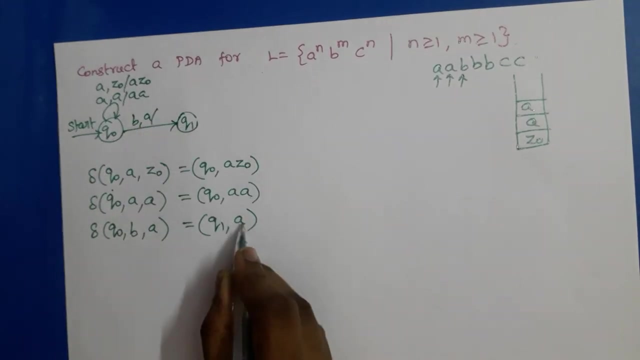 so we have to go to next state q1 and no change operation. No change means write the same a here, So don't do any operation with the stack q0 to q1.. It's just labeled by b comma a. slash this a. 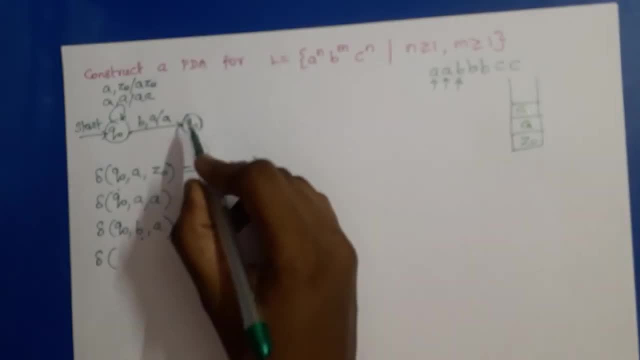 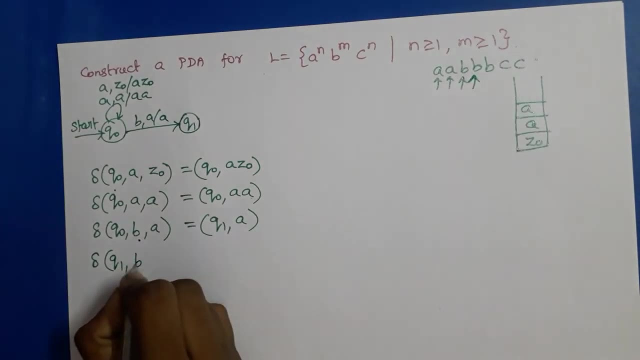 Then this is for one b. Now we need to write for the remaining b's, So q1 to q1,. we have to write So q1,. next input is b, Top of the stack is a and we should remain in the same state: q1 and no change in stack. 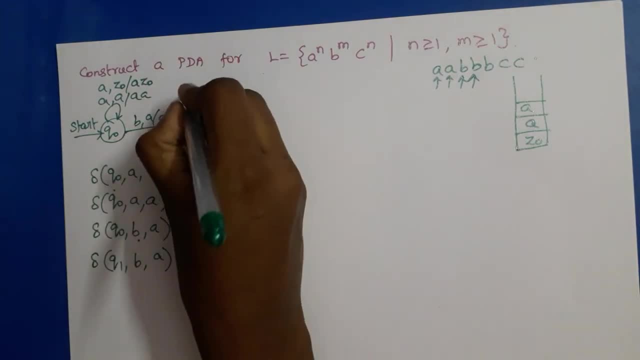 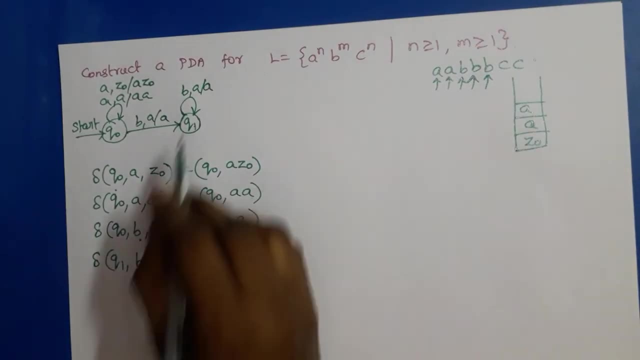 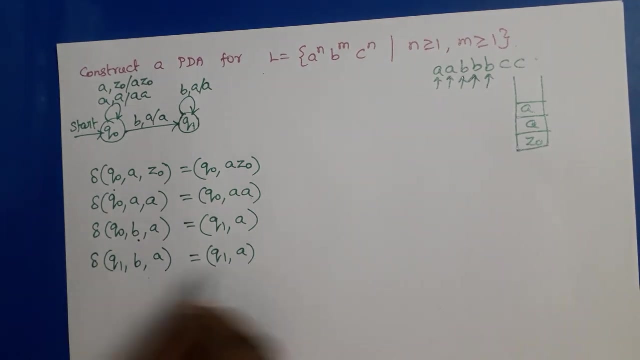 So from q1 to q1, b comma a. slash a should be written here, So the next input is also b and the current state is q1.. So q1 comma b comma a equals q1 comma a. So this is performed repeatedly for any number of b's. 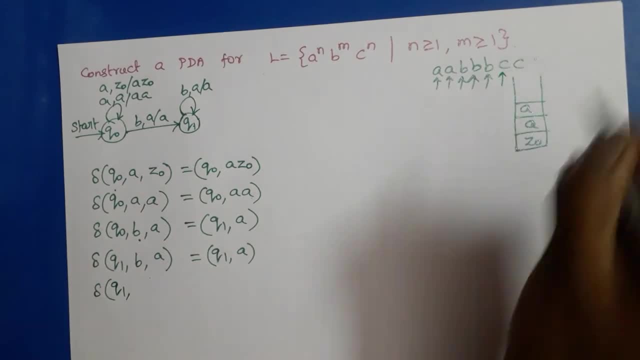 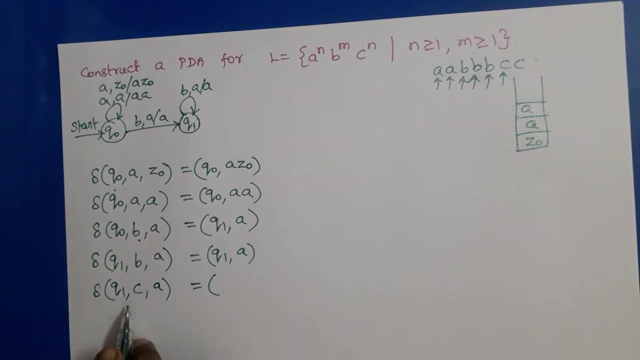 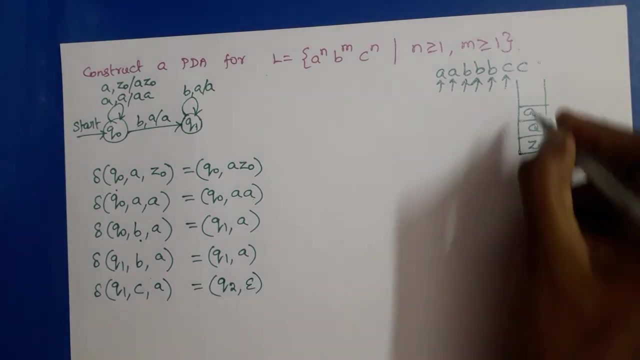 Next we are in state q1. And the current input c Top of the stack is a Means we have to pop one a right, So we need to go to another state. q2 and a should be popped from the stack. 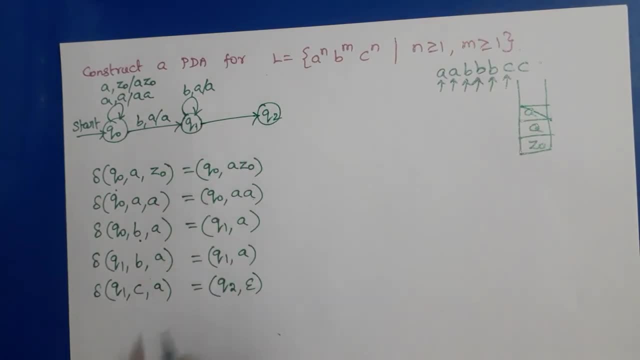 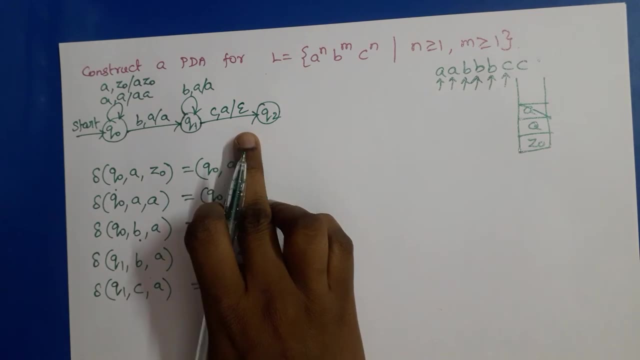 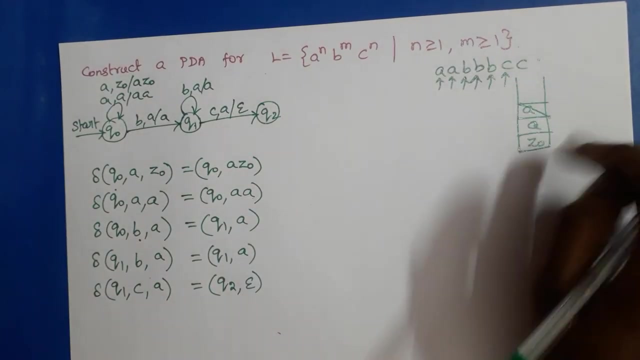 So q1 to q2, draw an edge and that edge is labeled by c comma a bar epsilon. This is for popping one a from the stack. Now the remaining c's, we have to perform the repeated pop operation. So delta of q2 is the current state. 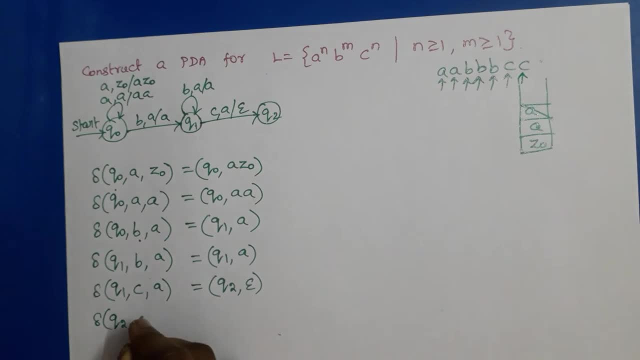 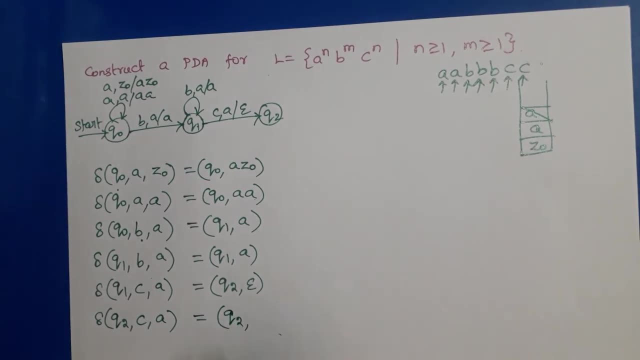 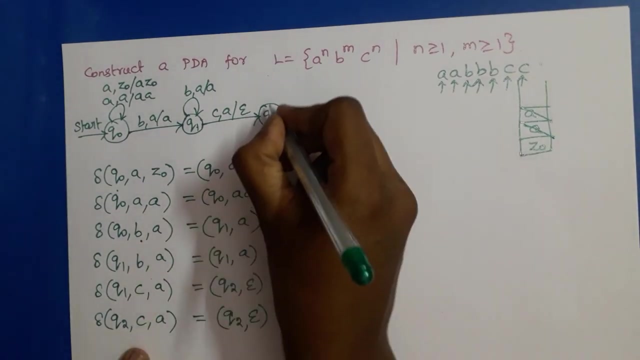 Now the current state is q2 and the next input is c. Top of the stack is a Means we have to remain in the same state- q2- and pop epsilon. So this is also popped from the stack. So q2 to q2.. 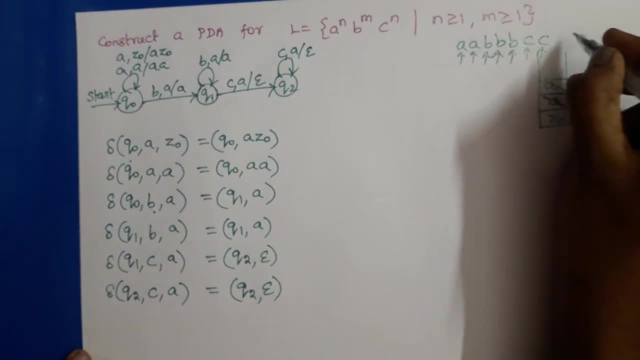 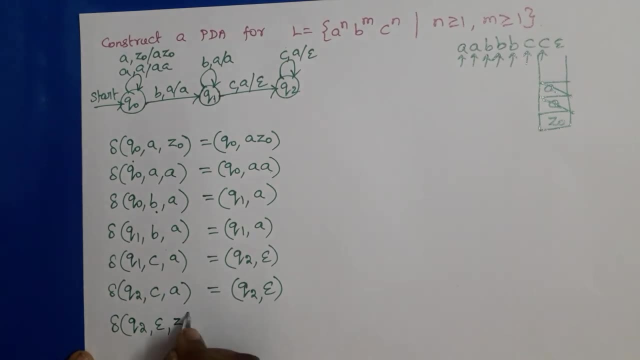 C comma, a bar epsilon should be written. So now the next input is epsilon, right. So q2 comma, epsilon comma. top of the stack is z. naught Means we have to go to the final state and we can empty the stack.